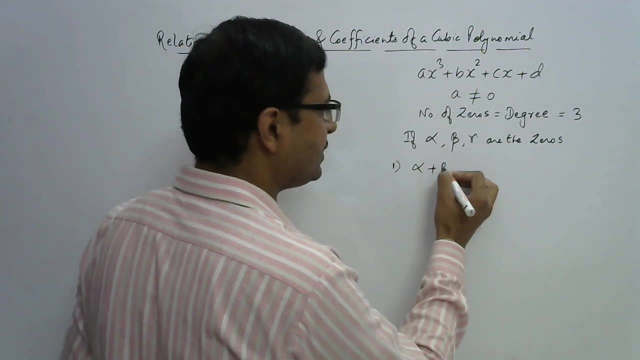 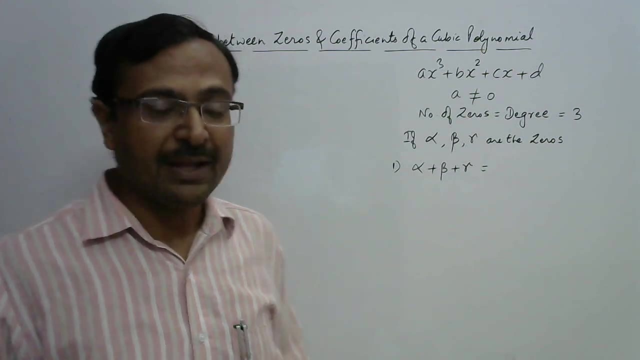 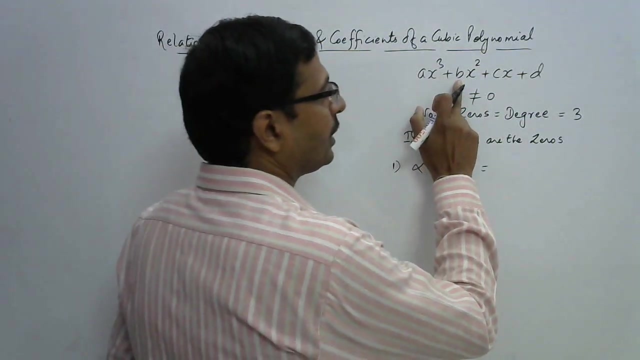 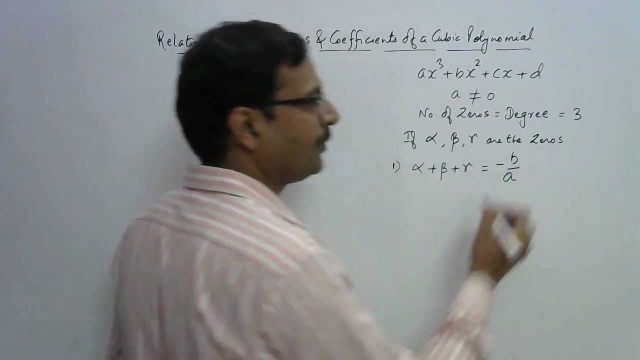 the sum of zeros, that is, alpha plus beta plus gamma, Whatever three values are the zeros of this cubic polynomial. if you find the sum of those three zeros, then that will be equal to negative coefficient of x square upon coefficient of x cube. Very important relationship, and so. 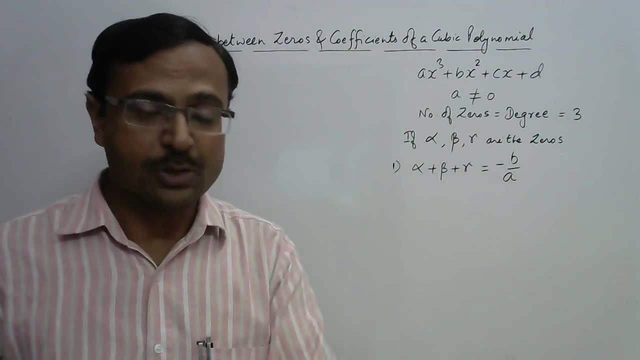 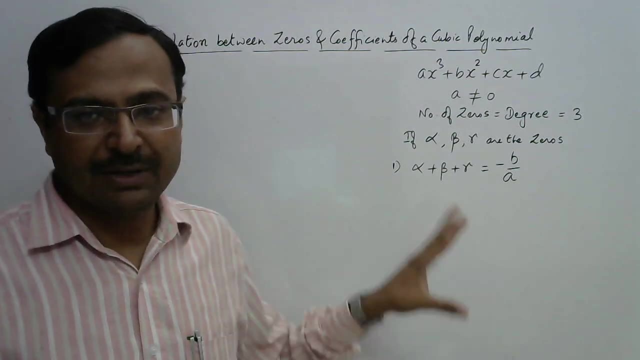 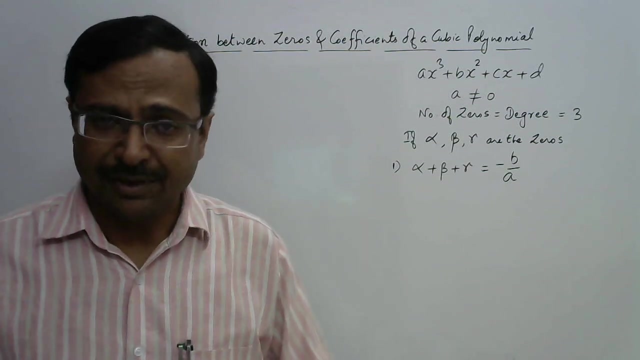 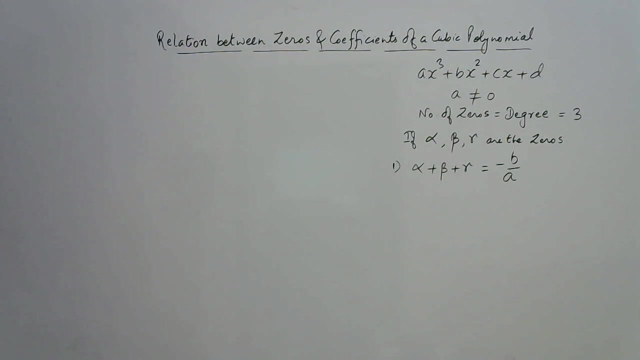 many problems are found in books. In class 10th also you have this topic and of the chapter and on polynomials, and in subsequent classes, obviously at competition level. these, this relationship between the zeros and the coefficients of the polynomial, are used in a wide variety of problems. This is the first relationship, that is the sum of zeros of a cubic. 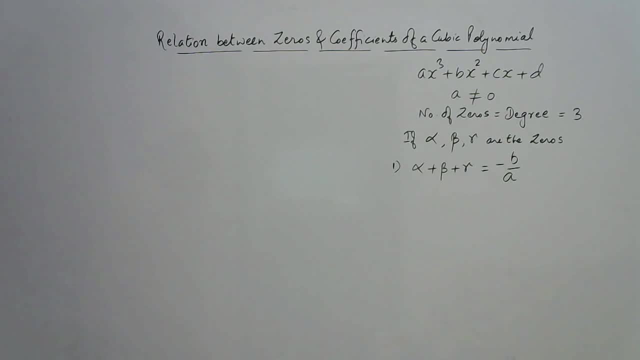 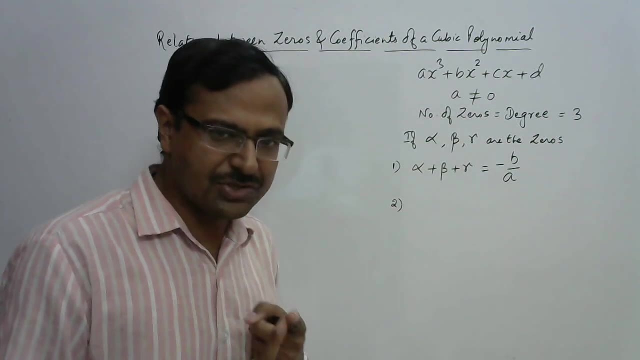 polynomial is always equal to negative coefficient of x square upon coefficient of x cube. Let us take the second relationship. In this relationship we will be taking the product of two zeros in pairs, like there are three zeros and there are five zeros, And if x is equal to x, 5 is. 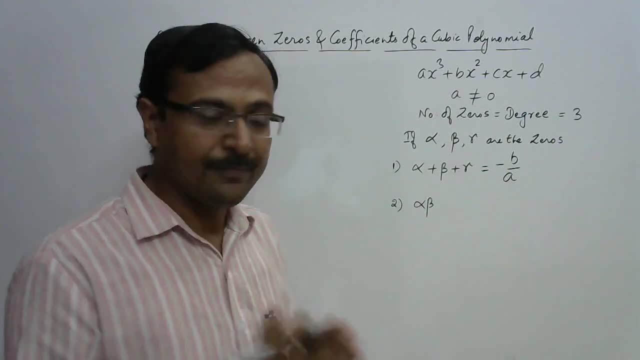 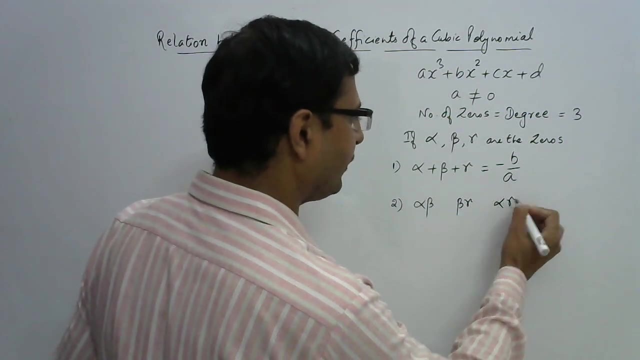 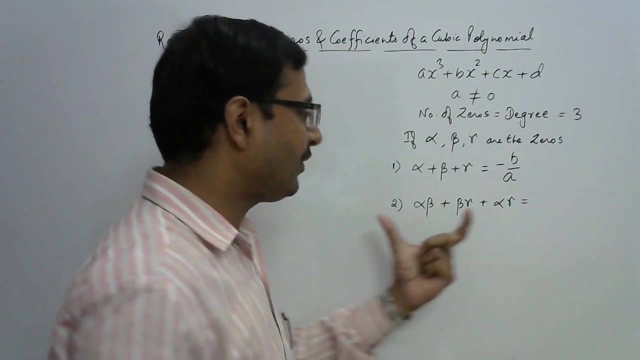 So we can add three products like: first is alpha into beta, Another one can be beta into gamma and the final one can be alpha into gamma. So if you take the product of the zeros in pairs and then add them, then this will always be equal to There. now there is a relationship between these and the zeros. 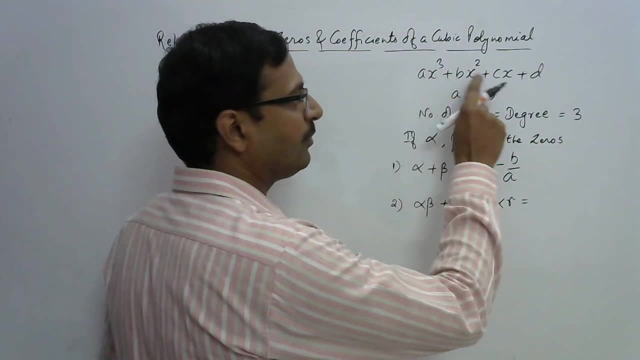 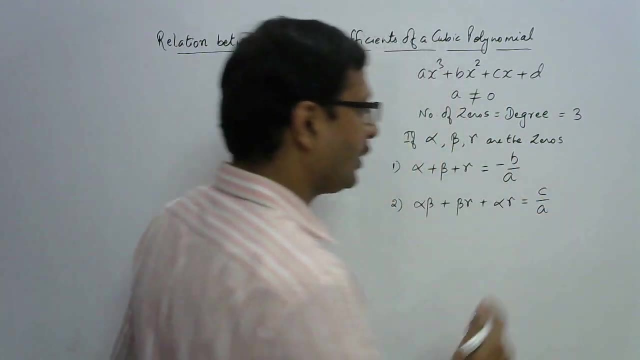 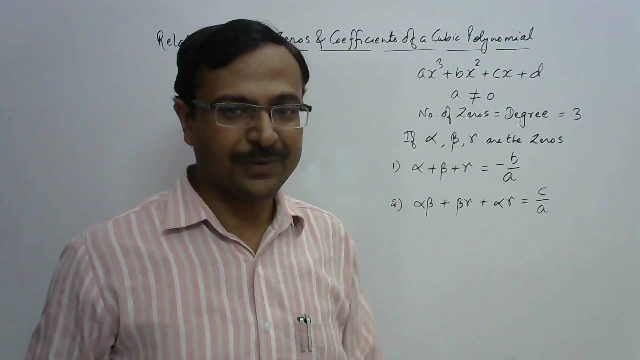 Now we started from here minus B by A. then we move from from B to C now, So it will be C upon A. So if the three zeros are found correctly, then this part will always be equal to C upon A and the final relationship, that is the. 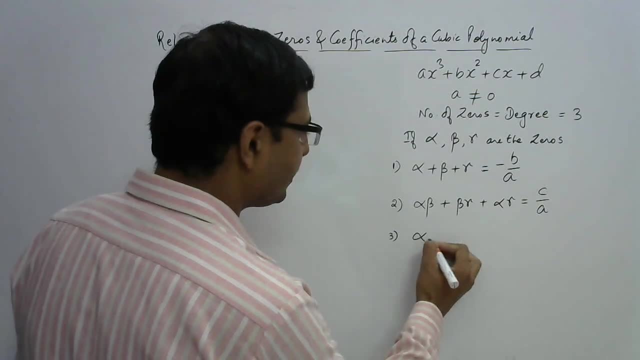 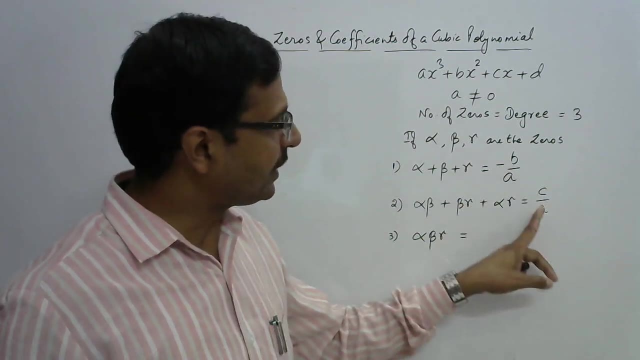 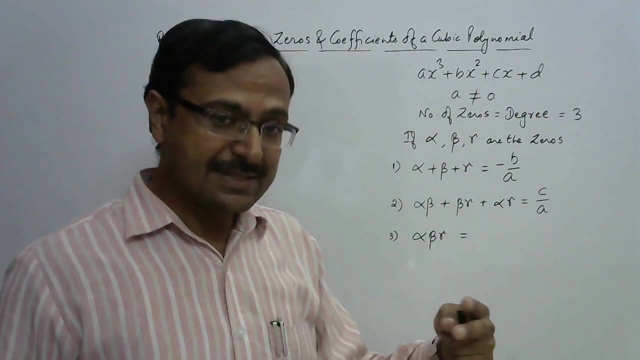 Third relationship is regarding the product of the three zeros, So alpha into beta, into gamma. See, we have taken negative here, then positive from B to C and now from C to D. So we move from C to B and again change the sign alternatively. so this is negative, this is positive. 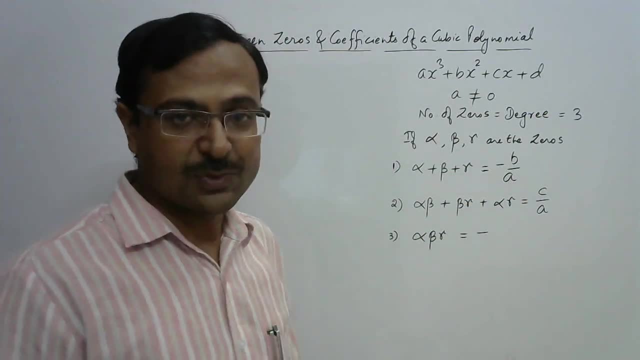 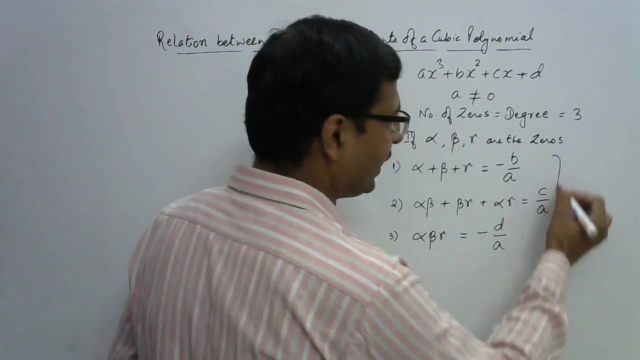 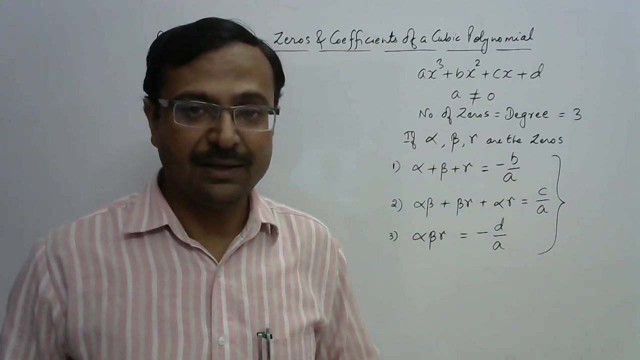 So now again we will have a negative sign, and this will be Constant term, that is D upon the coefficient of x cube. so in all the three relationships you find that the denominator is A, that is, the coefficient of x cube, and the sign will be negative for the first relationship, positive for the second and 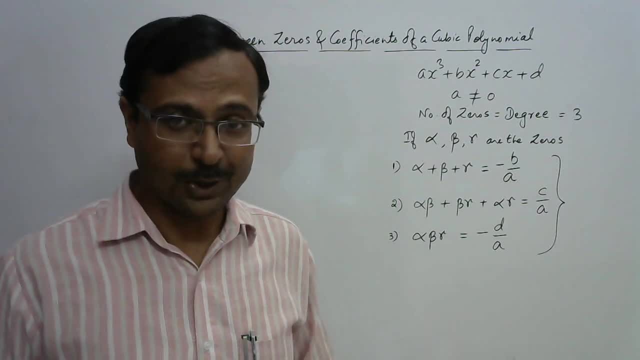 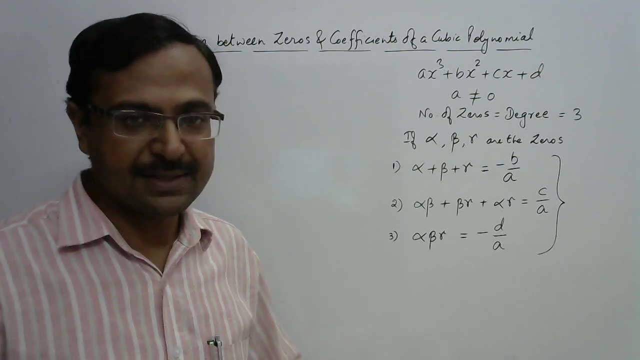 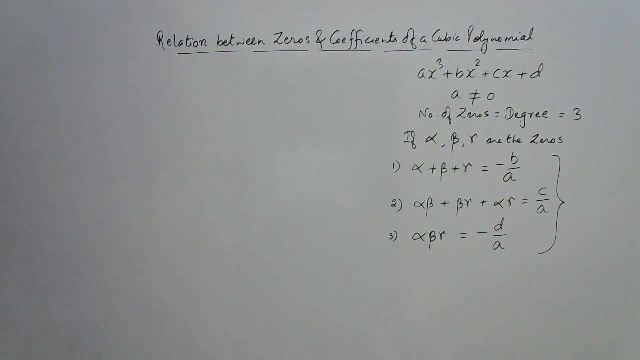 Again negative for the third relationship. Now this is the relation between the 0s and coefficients of a cubic polynomial. Now what kind of problems we get in exams- Let us solve one or two problems- and how we can use these relationships to solve those problems. Let us see the first one. Now there is a particular 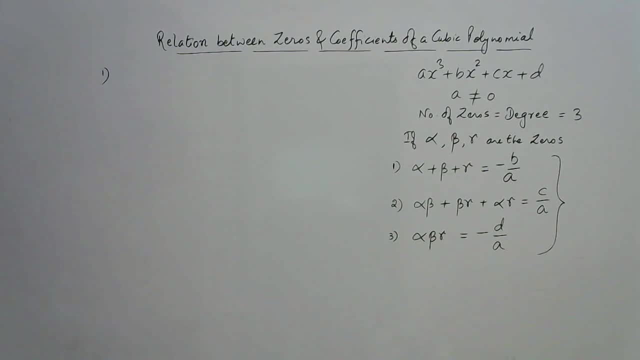 cubic polynomial which I am writing on the board. This polynomial is 6x cube plus 3x square, minus 5x plus 1.. So in the question it is given that if alpha, beta and gamma are its 0s. 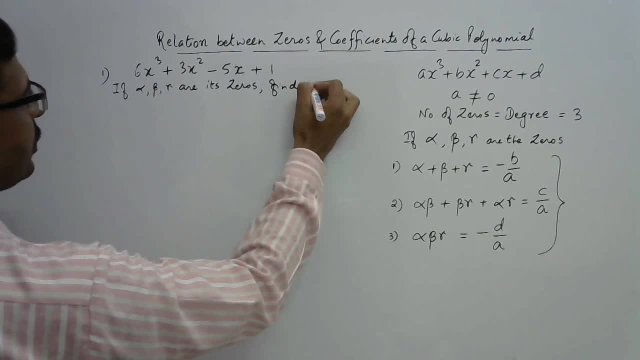 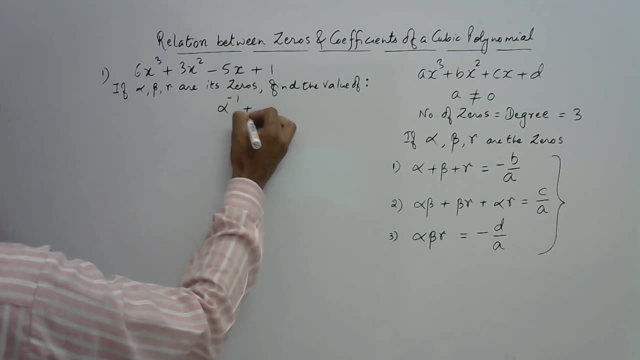 Then find the value of. so you have to find the value of a particular expression, and that expression is alpha power minus 1 plus beta power minus 1 plus gamma power minus 1.. Now you can find this type of question in your class 10th books, also in the chapter on polynomials. 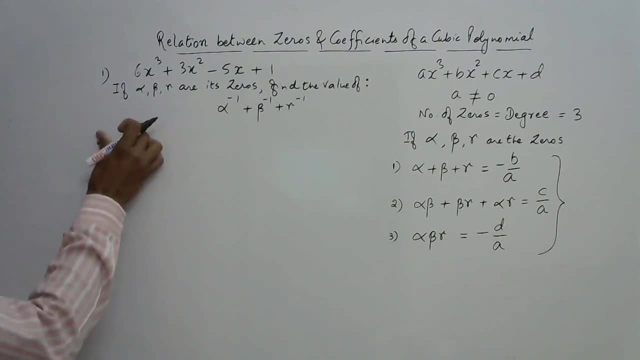 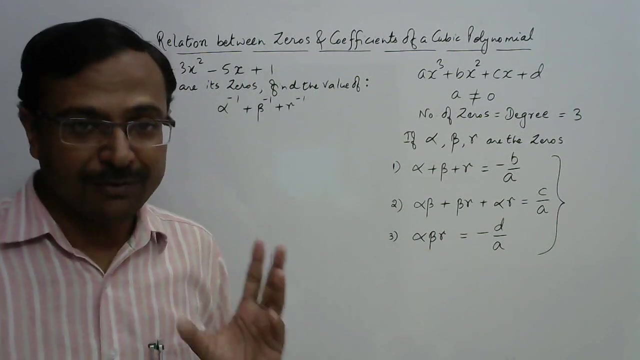 So how do we solve these kind of problems? Now see, in this problem, the first thing we must understand here is the three 0s of this. cubic polynomials are not to be found out, because that itself is a lengthy process. Solving a cubic polynomial will take a lot. 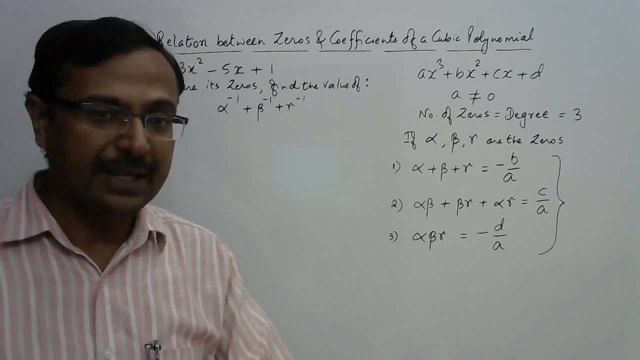 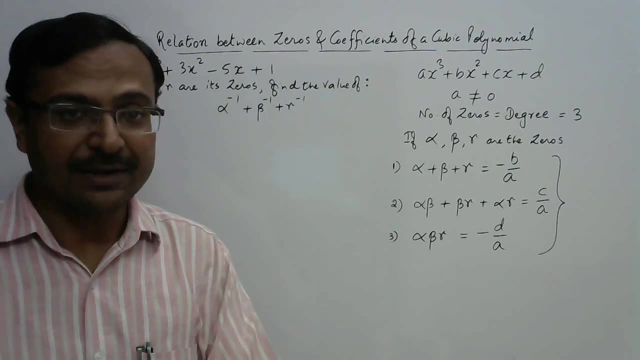 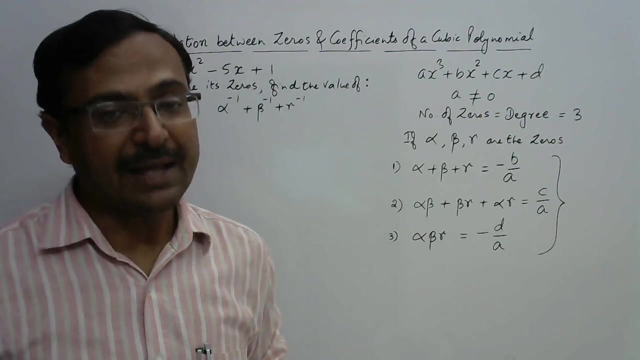 of time if you are not aware of the correct method, because the only method which is taught for solving a cubic polynomial to get the three 0s is the trial and error method or the hit and trial method, which the students study at class 9th level. But if you start, 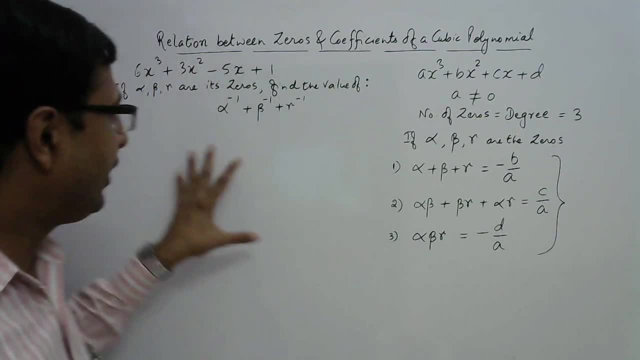 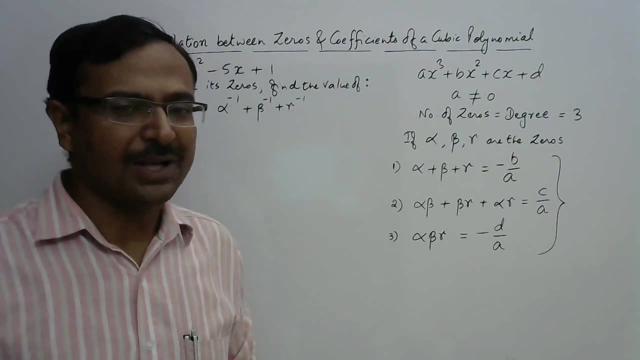 with the hit and trial method, then obviously this problem will take a lot of time. but if you know the relationship between the 0s and the coefficients then this problem can be solved hardly in, say, about 15 seconds time. Let us see whether we can do that or not, Because 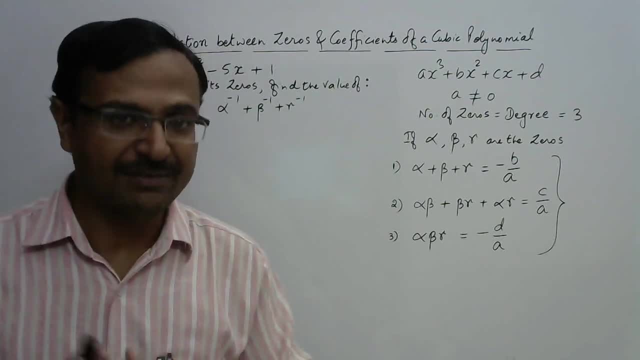 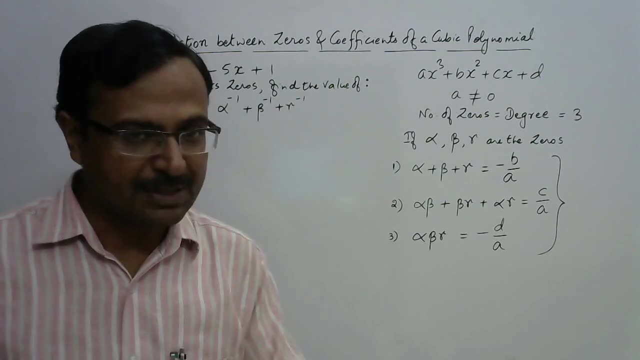 I will take more time just because I need to explain each and every step to you. And once you are well acquainted with the steps, then the timing of 15 seconds can be achieved with the practice of 1 hour. So let us see how this works. 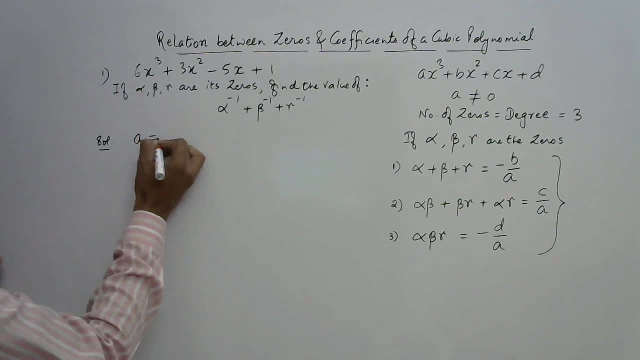 this can be done Now. in this case, the coefficient of x cube a is 6. here, then, the coefficient of x square, that is, b, is 3, coefficient of x is minus 5 and constant term is 1.. So the first thing is I need to find a, b, c and d from the given cubic polynomial, and after this I will make use of: 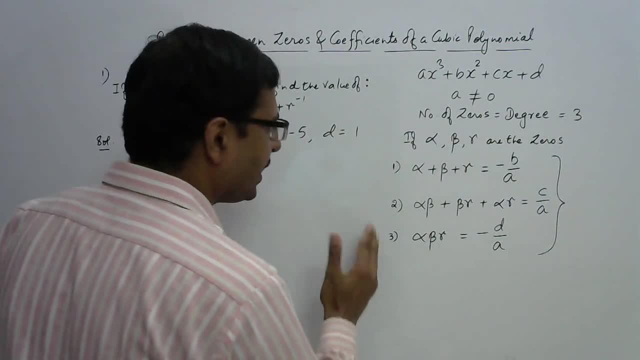 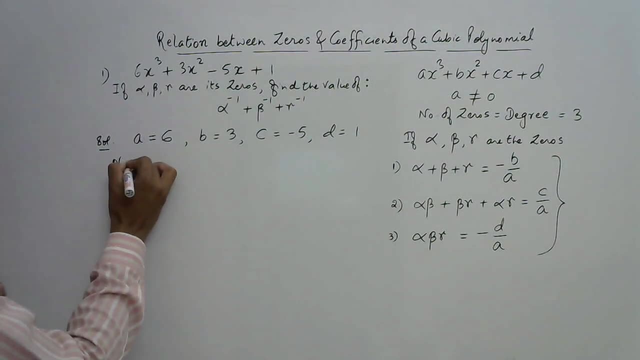 the relationships. whatever relationships I need, I will use only those relationships. I will not write all the three. Now we have to find the value of alpha power minus 1 plus beta power minus 1, plus gamma power minus 1, and power minus 1 means reciprocal, so this is actually 1. 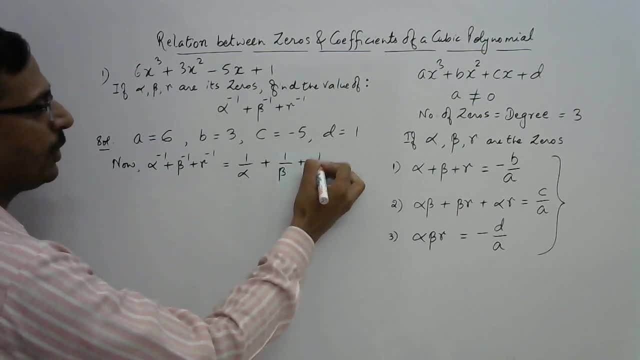 upon alpha plus 1 upon beta, plus 1 upon gamma. and if you take LCM of these three terms, you will have alpha beta gamma and you will have alpha beta gamma and you will have alpha beta gamma and the denominator and in the numerator alpha is already there, so you have beta gamma plus so beta. 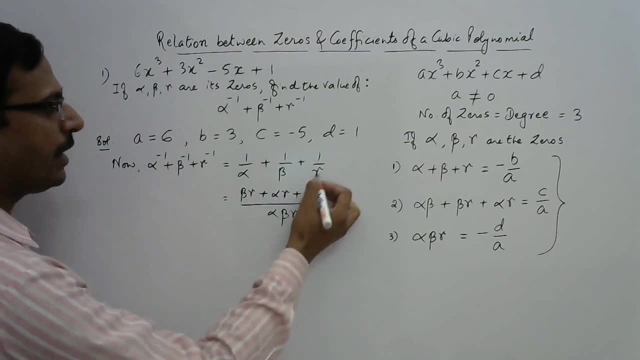 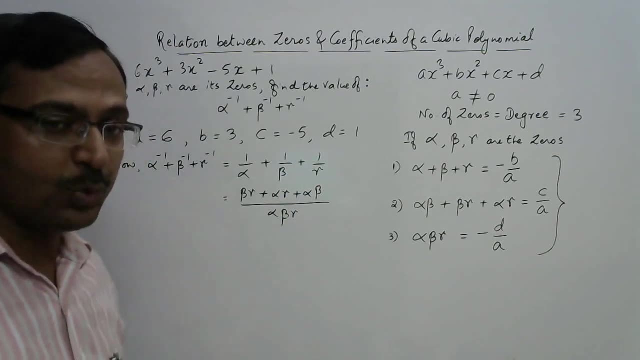 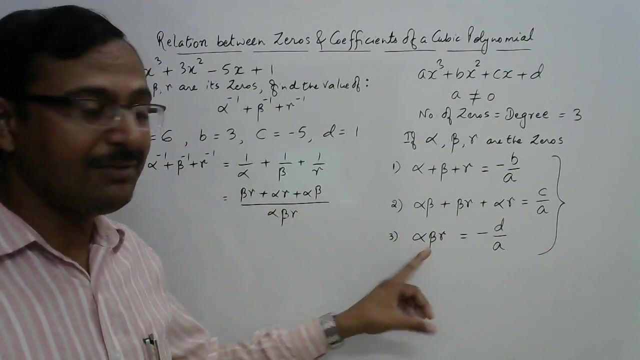 is already there means alpha gamma, and gamma is already there means alpha beta. and now this expression gives you a hint that we have to consider only the relationship number 2, which is in the numerator here, and the relationship number 3, which is in the denominator. So I can. 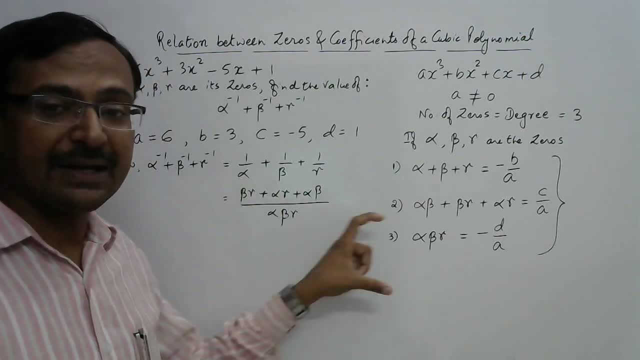 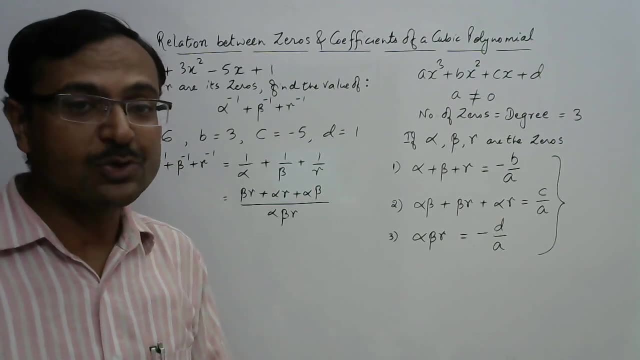 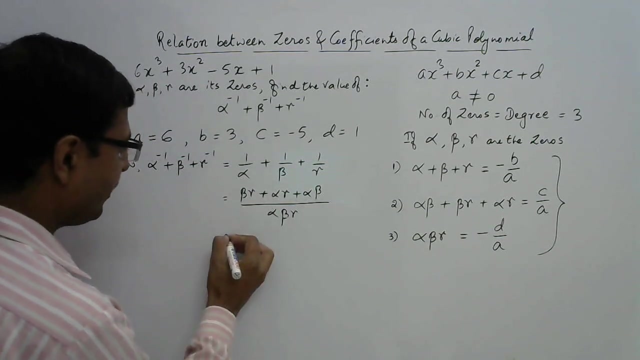 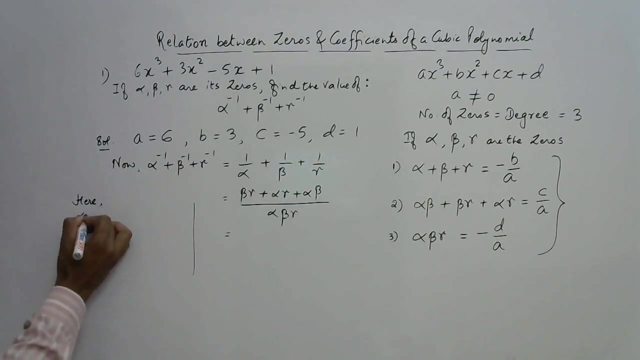 find the values of this numerator and denominator directly by using these two relationships and just substitute the value here to get the desired answer. so I don't need the values of alpha, beta and gamma separately. so let us see how that value can be found out. see, I'm solving it here here. alpha, beta plus beta, gamma plus gamma: alpha is: 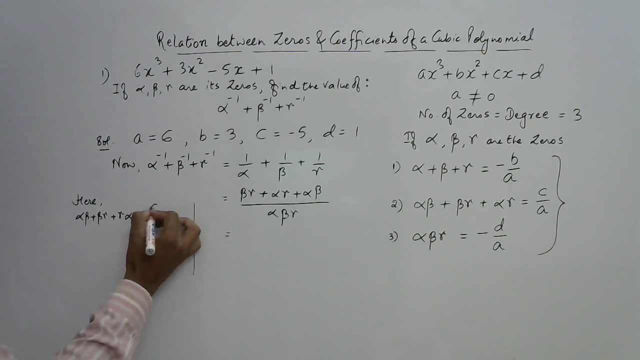 see the relationship get the c upon it in the numerator as minus six, false. thus we have a value of the numerator as minus 6 and I'm already written the values of ABCD here. so c upon c is minus 5 upon a is six. so we: 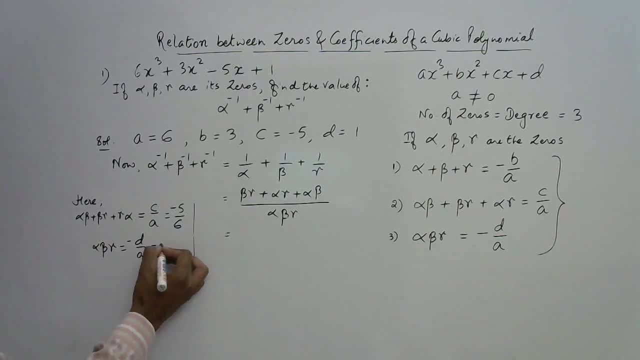 have the value of the numerator as minus 5 by 6. similarly the denominator alpha beta gamma. the formula for alpha beta gamma is minus d and once you have the formula, just substitute the values minus d. what is d, d is 1 and a is 6. so see, I have already written the values of alpha beta and gamma plus alpha beta minus a. plus a is minus 4. so give it in the numerator. 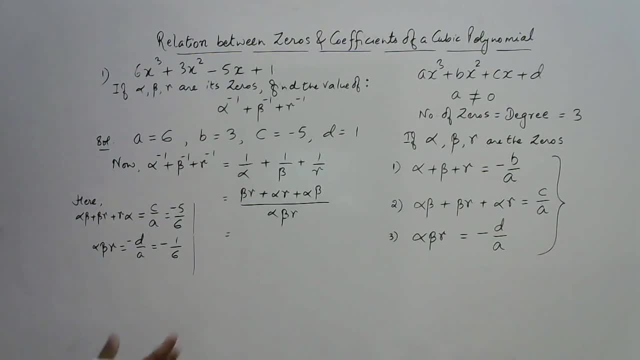 both the values now And in the next step. the answer is there. Numerator: the value is minus 5 by 6. And denominator, the value is minus 1 by 6.. This comes out to be minus 5 by 6 into minus 6 by. 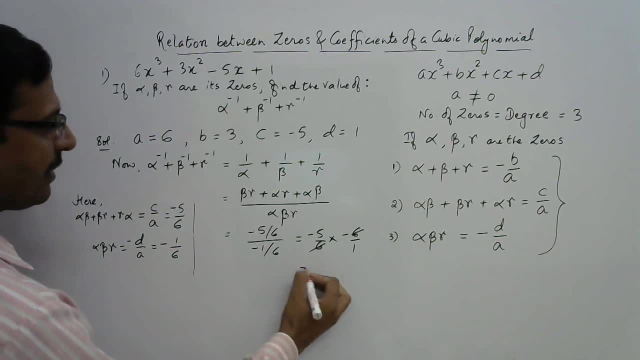 1. So 6 gets cancelled, thereby giving you the answer. Minus, minus is plus, So you have the answer 5.. So the value of this expression is 5.. A very easy question if you really know the. 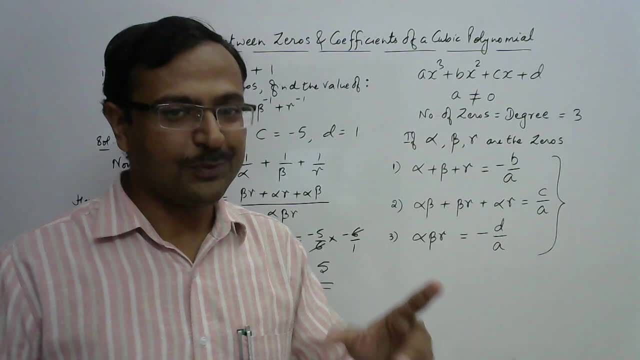 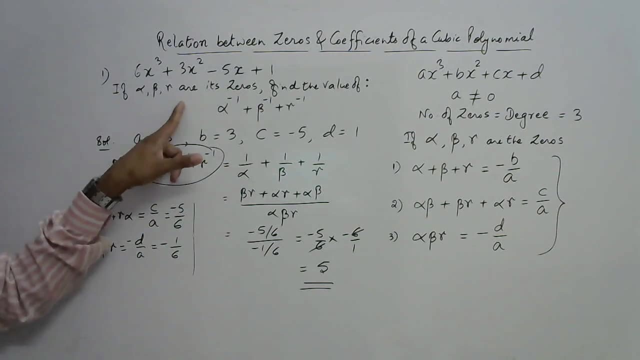 relationship between zeros and the coefficients of the polynomial. But if you are not aware of this, then you will be struggling to find out the values of alpha, beta and gamma by using intent trial method And that will consume a lot of time also, But the answer you know. 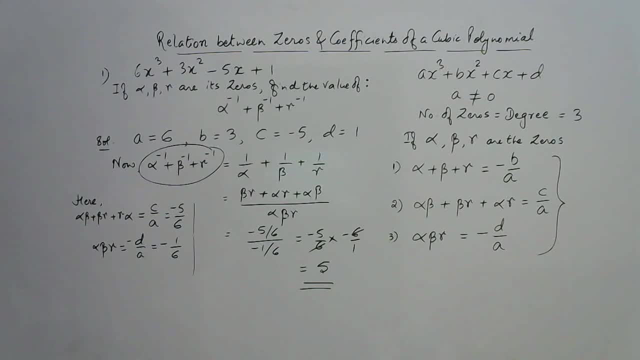 that is also not guaranteed. So these type of questions are very prevalent in competitions, because actually this is based on the knowledge of the relationship, not on how you know the roots are found. It is based on the relationship between the zeros and the coefficients. So, friends, learn all these. 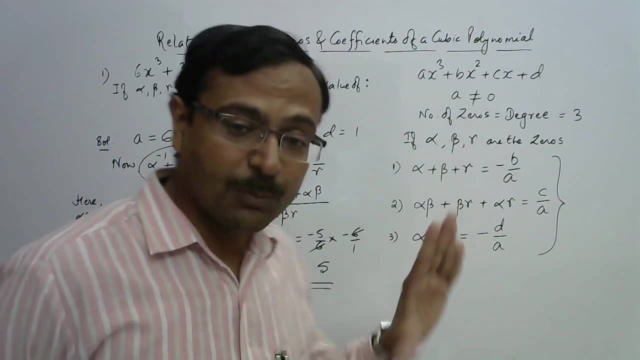 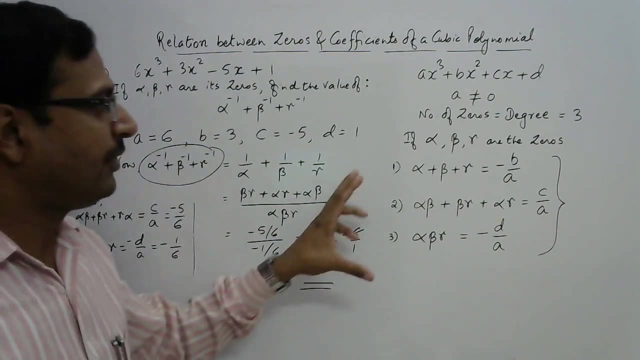 methods. We shall practice this concept, taking more examples in subsequent time. Till then, if you like this video, please subscribe to our channel. Thank you, And you have understood this method of solving questions related to alpha, beta and gamma- that is, the three zeros of a cubic polynomial- And share it with all those friends who are 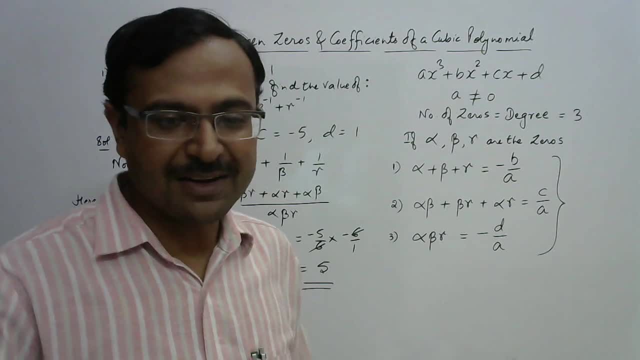 appearing in board exams this year, And do not forget to subscribe to the channel for more such useful videos to come in future also.